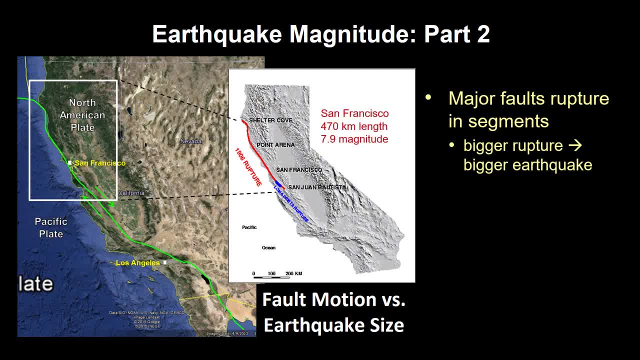 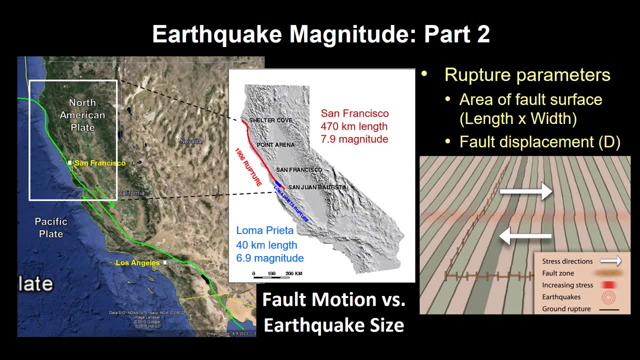 ruptured a segment of the San Andreas that was 10 times longer than the break caused by the 6.9 magnitude Loma Prieta quake. To get an accurate measure of earthquake magnitude on these larger fault segments, we must be able to constrain both the area of the fault. 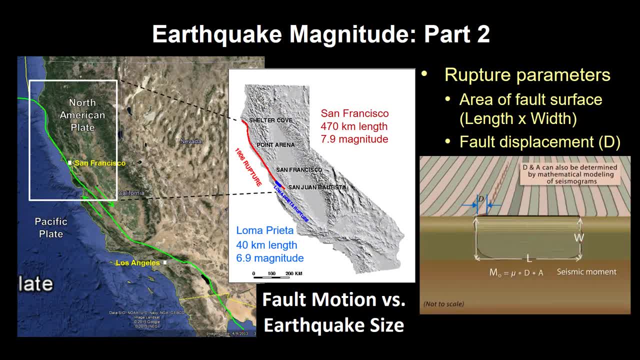 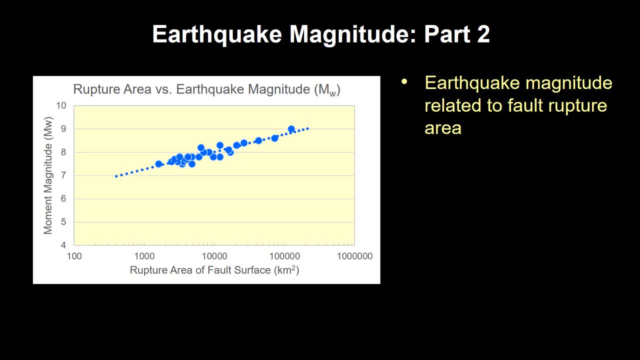 that ruptures and the amount of fault displacement. This graph plots the rupture area of certain earthquakes of magnitude 7 or greater against earthquake magnitude. If all else were the same, rupture area alone might be sufficient to allow us to estimate magnitude. However, 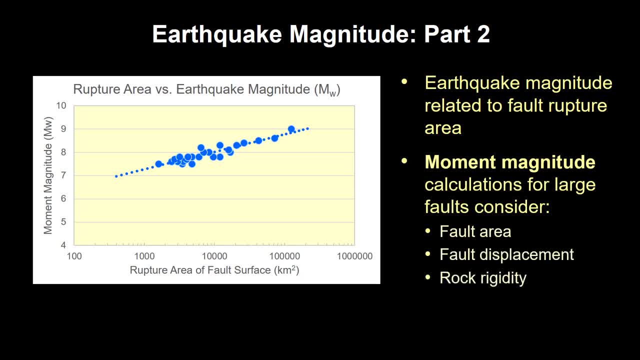 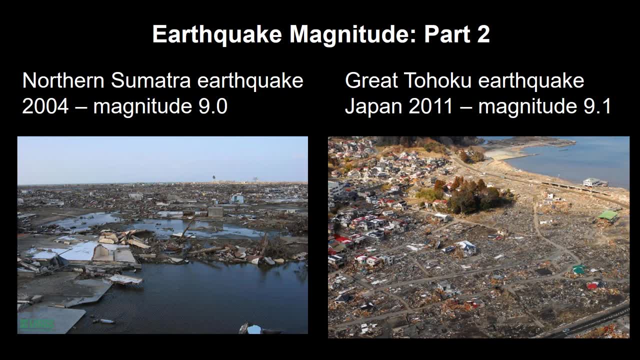 additional factors such as the amount of fault, displacement or the rigidity of the surrounding rocks can also be significant in determining earthquake magnitude. For example, two mega earthquakes of similar size both occurred on subduction zones and resulted in widespread devastation. The Northern Sumatra earthquake featured a large rupture surface and a significant amount. 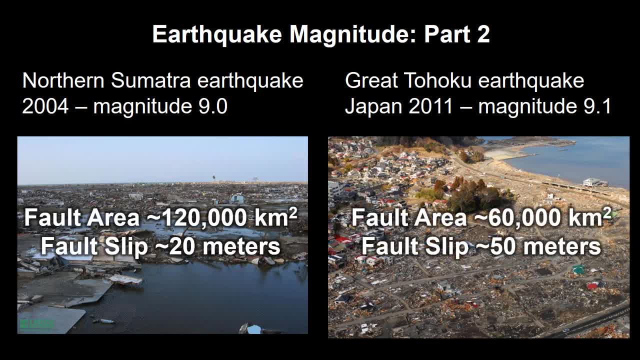 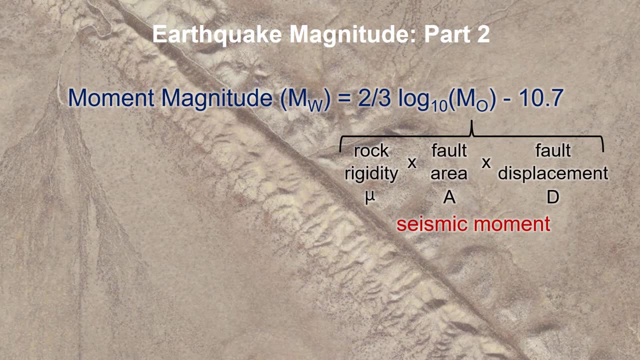 of fault slip. In contrast, the Tohoku earthquake compensated for a smaller rupture area by generating more fault slip than had ever been recorded for any other earthquake. The rupture area, displacement and rigidity contribute to a value known as the seismic moment. Geologists, or really super-fast computers, plug this seismic moment value into an equation. 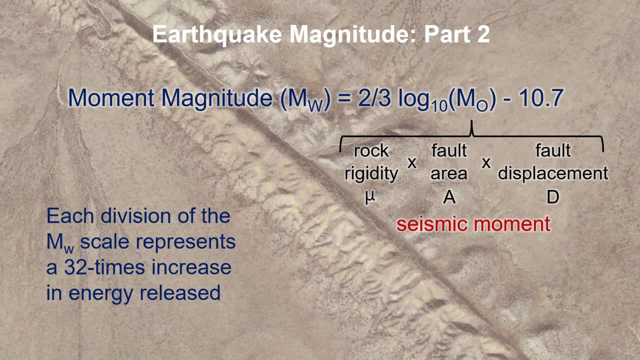 to determine the moment-matter ratio. This is the value that gets reported when you read about big earthquakes in the news. Not only does the recording on a seismograph increase in size by 10 for each step-up in magnitude, but the energy released by the earthquake increases 32 times. 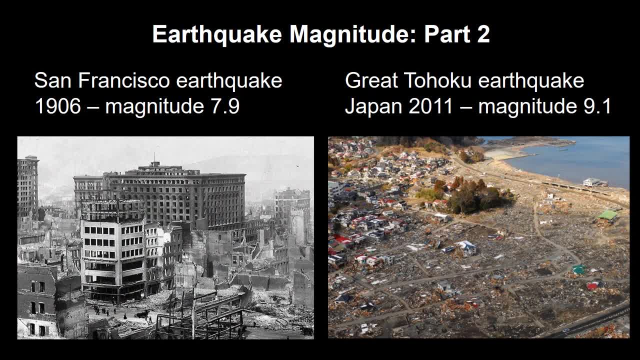 For example, let's compare the 9.1 magnitude earthquake in Japan with the 7.9 magnitude San Francisco earthquake. The earthquake in Japan would have been nearly 16 times larger on the seismograph record and would have released 63 times more energy. 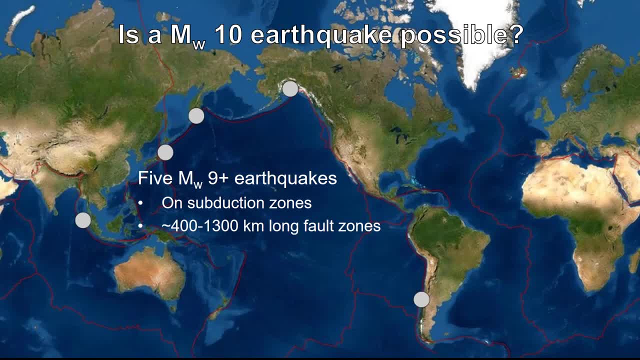 This is the seismic record we used to determine the magnitude of the earthquake, and now it's Since 1950, there have been just five earthquakes of magnitude 9 or greater recorded around the world. Each occurred on a subduction zone along a convergent plate boundary. 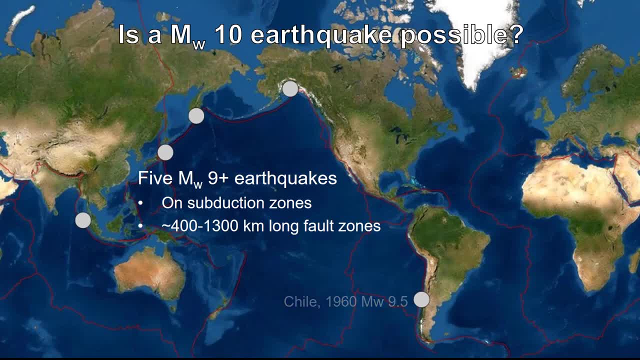 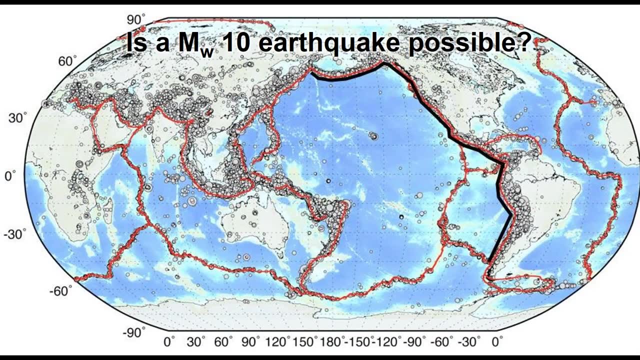 The biggest of these was a magnitude 9.5 earthquake in Chile. Could a magnitude 10 earthquake be in our future? Well, no. To get a fault big enough to generate a magnitude 10 earthquake, you'd need something like this: a 14,000 km long boundary. 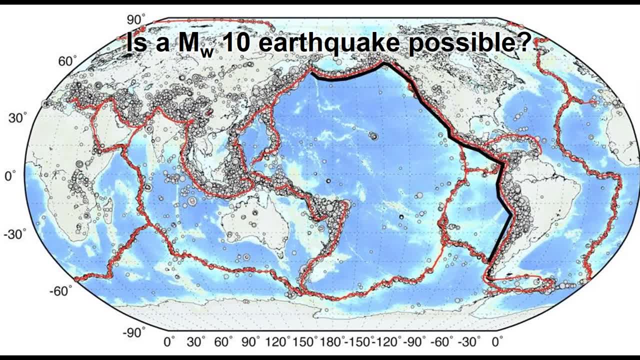 that would link together multiple fault systems along the margins of the Nazca, Cocos and Pacific plates, And that's probably just not realistic. The energy produced by an earthquake is a pretty abstract concept, but the damages of the result are real and can be readily observed and experienced. 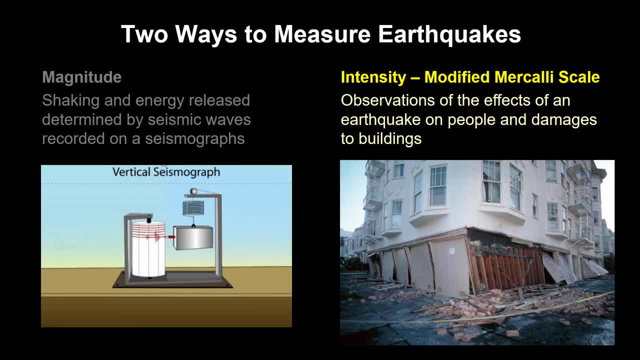 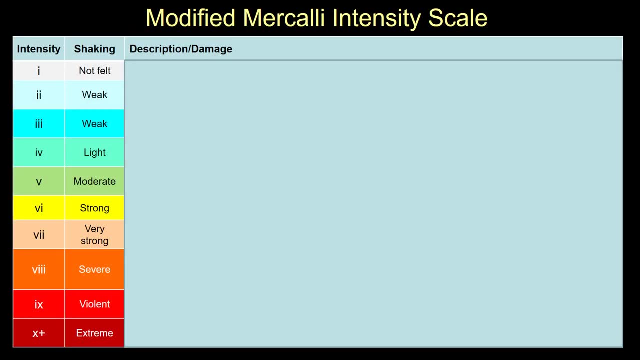 by millions of human beings each year. We label this the earthquake intensity, and it's measured using the modified Mercalli scale, which focuses on the effect an earthquake has on people and the damage that might occur. The Mercalli scale has 12 categories, represented by Roman numerals. 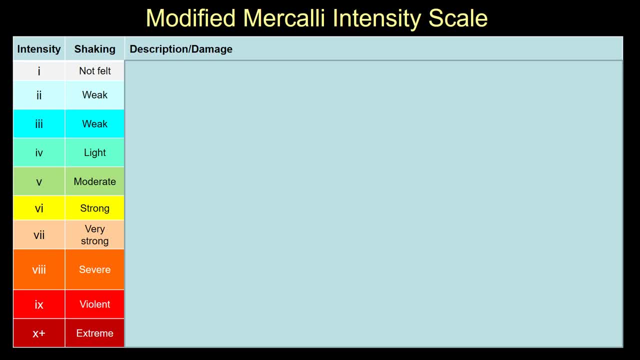 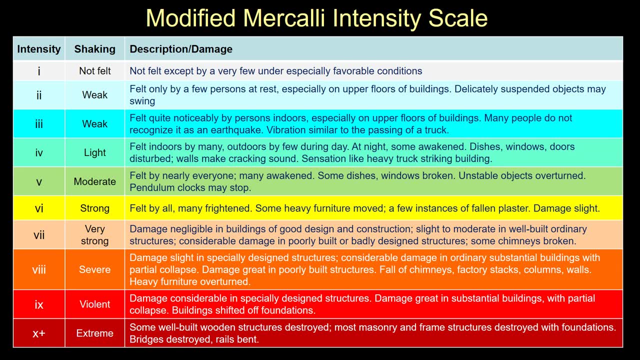 We've grouped the last three categories together as their characteristics often overlap. Each category has a brief description to help the application of the scale. Don't expect to remember all of these details, Just be aware of the general trends. For example, the first two categories represent: 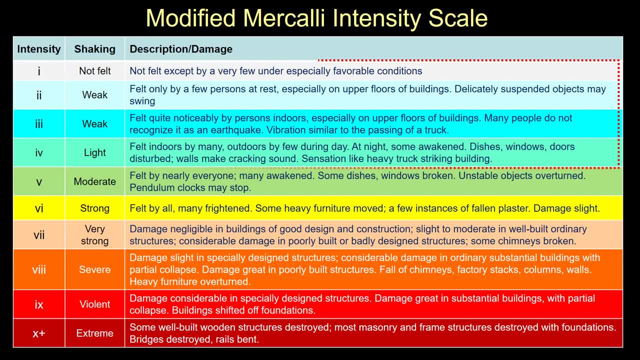 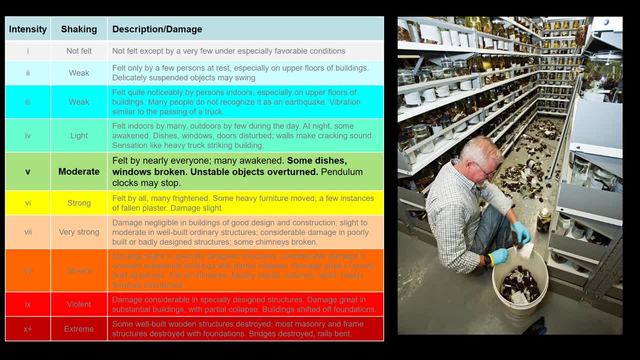 relatively minor damage and have relatively little or almost no effect on people. For example, the first two categories represent relatively minor damage and have relatively little or almost no effect on people. Things start to get more interesting. around intensity five You'd certainly know that you were in an earthquake, And if you're, the Smithsonian Museum. 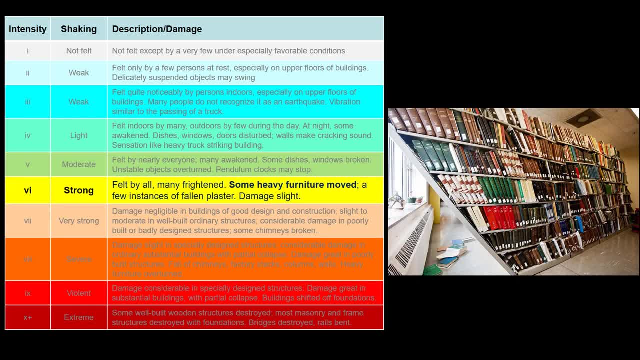 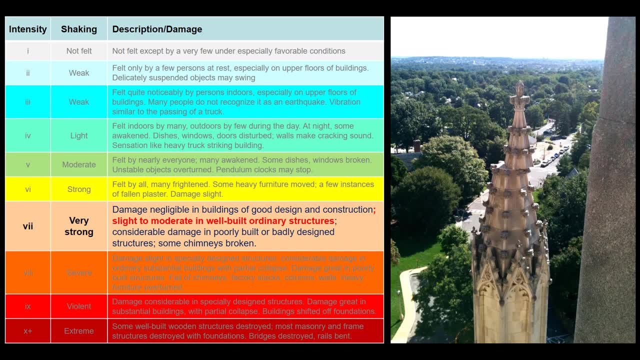 your collection of preserved specimens might suffer some damage. At intensity six, unsecured heavy furniture gets moved around. Maybe those bookcases fall over At seven. unless you're living in a building that's engineered to deal with earthquakes, chances are you'll start to see some evidence of damage. 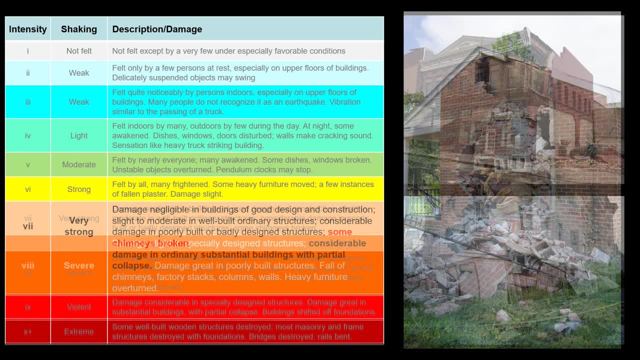 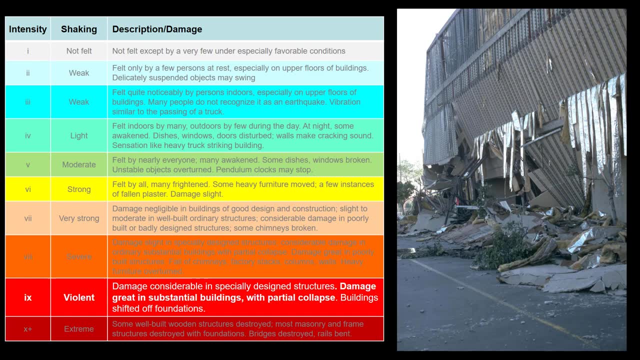 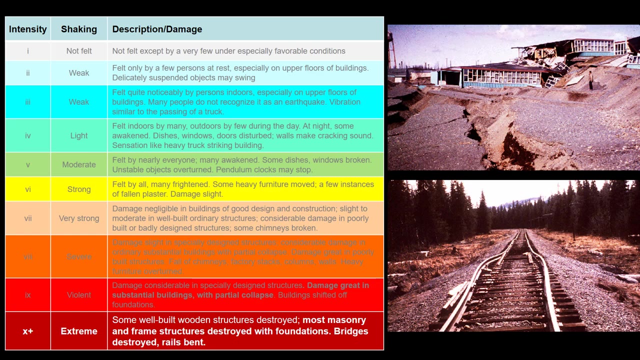 often represented by collapsed chimneys. At category eight, we're seeing substantial damage to many buildings, some of which may partially collapse. Damage gets even more significant and wide-ranging as we continue to higher levels on the scale. We see whole buildings and other structures collapsing. 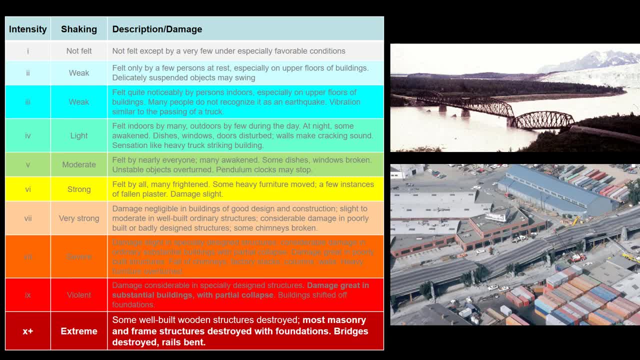 potentially resulting in multiple deaths and injuries. Because the damage varies with distance from the earthquake and with a variety of local factors, there will be multiple intensity values for any given earthquake. Intensity values will be higher and more wide-ranging for larger earthquakes.